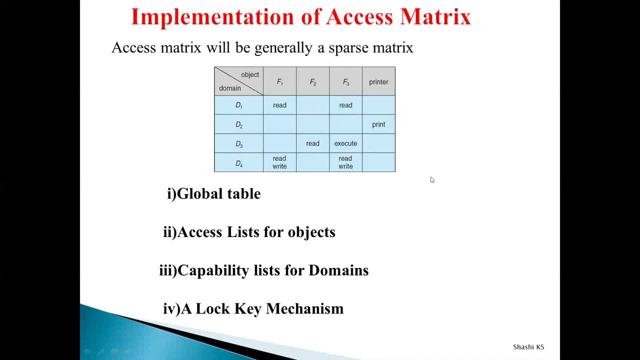 and the actual protection policy will be implemented. Okay, so that is what we learned about what is an access metrics in the previous lecture. So in today's lecture we will see about the different implementations of fabricis matrix. As I told you before then, this question is asked in the examinations, if they ask you. 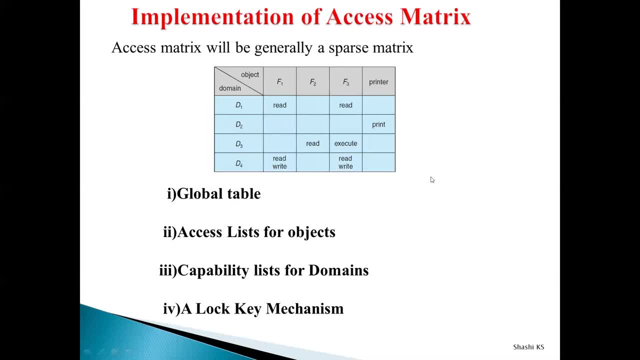 to write in the right about access metrics with examples. you have to write about what is access metrics and what is the representation, what are all the information which will go into the access metrics. But then if they ask you to write the information and then you have to write all the information, 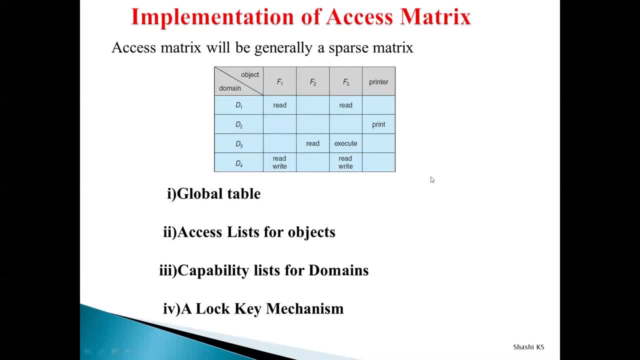 about implementation. you have to write about what are all the different data structures by which you can implement this access matrix. so, generally, while talking about implementation, if you see the access matrix, this is how your access matrix will look: like row wise: it consists of domains and the columns consist of objects. what do i mean by objects? objects are nothing but the resources. 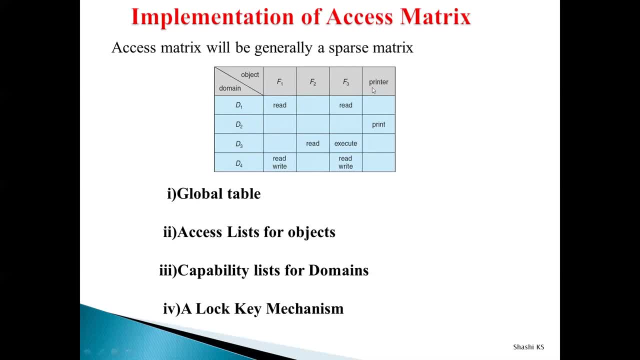 it can be anything like your, it can be a hardware object or it can be a software object. it can be hardware object, like the cpu or the or the magnetic disk, or it can be a software object, like a file or your semaphores, etc. so then in the rows, the access matrix consists of domains. so what is? 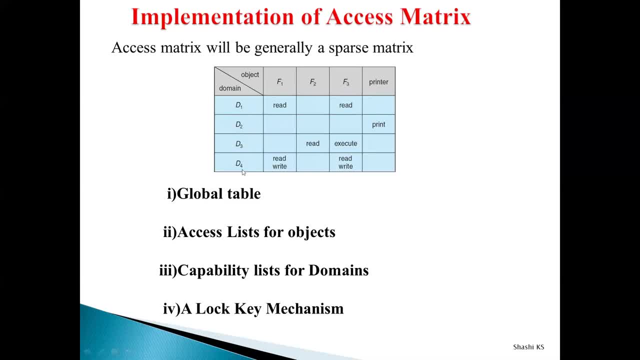 the meaning of domains. domain is nothing but every process is set to operate on a domain. and what is the meaning of domain? domain is nothing but the set of resources which a process can access. okay, so if you have a domain, domain is set to be a domain. so this is how generally your access. 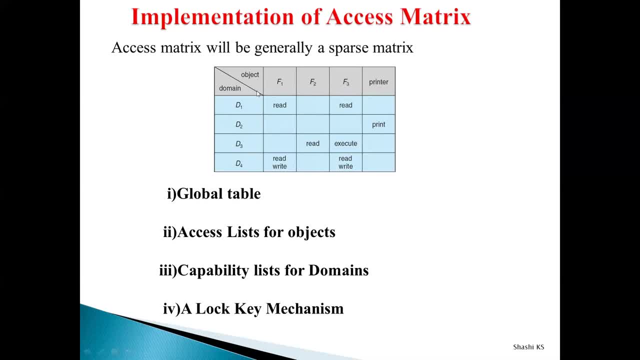 matrix will look like. okay, just try to observe this representation of access matrix, because then only you can understand its implementation. okay, so rows in the access matrix consist of domains. domains are nothing but the set of resources which a process can access, and the columns of an access matrix consist of objects. objects are nothing but the resources which can. 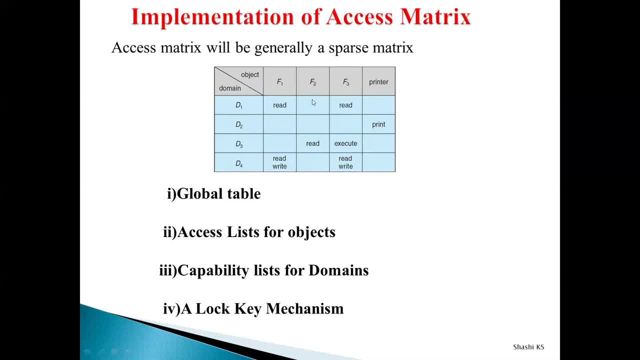 be a domain domain or it can be a software resource. and what is the entries of the access matrix on the stock? the entries are called as access rights. so access rights are nothing but the operations which can be performed on that particular object in that particular domain, say, for example. if you want to, if say, for example, a process in domain d1 can perform read operation, 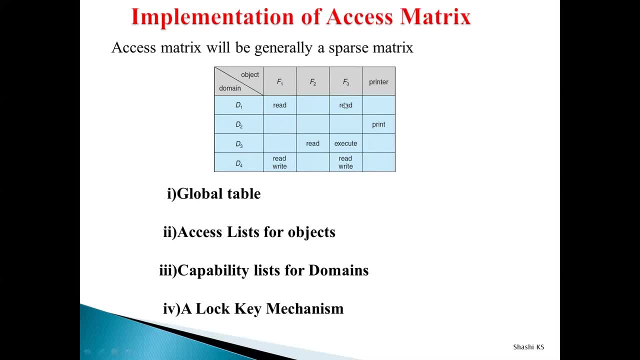 on the file f1 and it can perform read operation on the file f3 not allowed. that is the meaning of this representation. similarly, a process in domain d2 can perform print operation on the printer resource. that is the meaning of the second row of this access matrix. so that is the meaning of the general representation and the 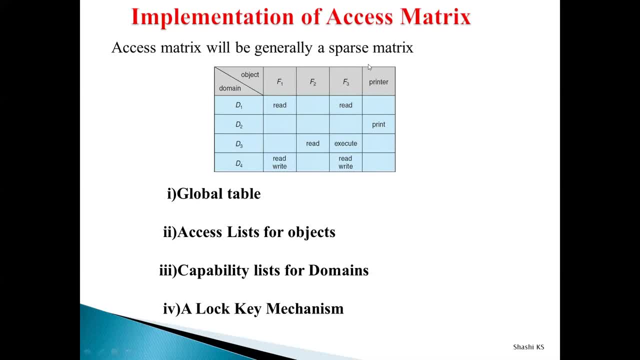 meaning of the access matrix, and this access matrix is generally a sparse matrix. what is the meaning of sparse matrix? sparse is nothing but a matrix in which most of the entries are empty entries or zero entries. most of the entries will be zero, zero or empty entries. 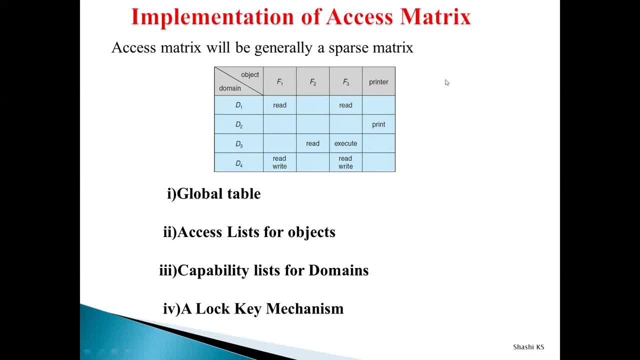 So nowadays, we make use of this sparse matrix implementations in machine learning and natural language processing for processing data. So, though we have a lot of data structures to implement this sparse matrix, you can use a array or you can use a link list to implement this sparse. 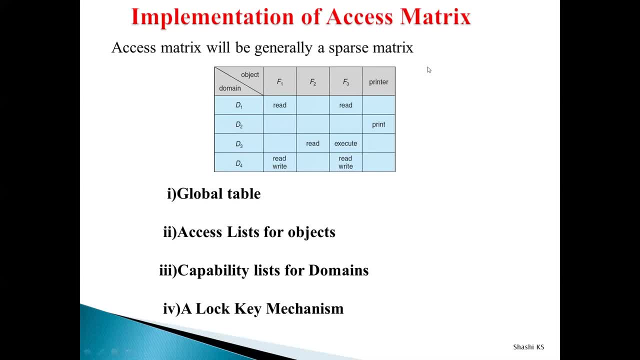 matrix concept, but then it will not be able to implement our concept of protection. So that is why all the existing implementations of sparse matrix cannot be used to implement this access matrix concept for our protection. So for that reason we have four different implementations for implementing the access matrix. 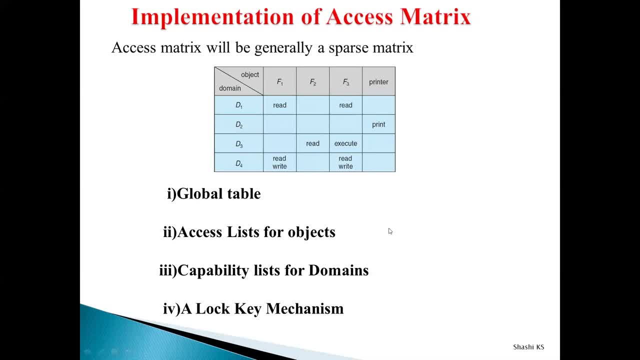 So there are four types of implementations. Also note that this is a very important question which is frequently asked in all university examinations. Okay, There are four types of implementations for access matrix. They are listed here. First implementation is called as global table. 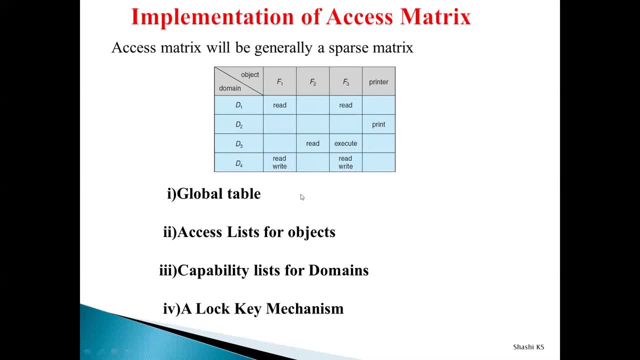 Second implementation is called as sparse Access lists. Third implementation is called as capability lists. and the fourth implementation is called us lock key mechanism. Okay, So let's see about each of these implementations in detail before going into the implementation. Just try to understand this representation rows of the access metrics consists. 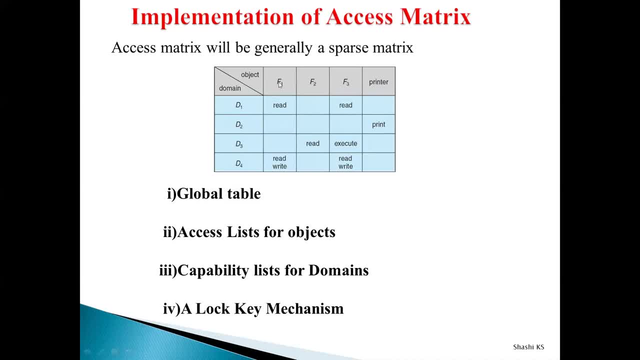 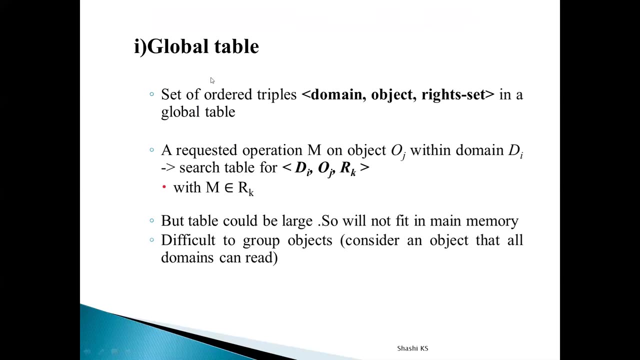 of domains and columns of the access metrics consists of resources and each entry in the access metrics is set to consist of access rights, which is nothing but the operations which can be performed On the object. Now let's go into the implementation. So first, implementation of your access metrics is called as global table. 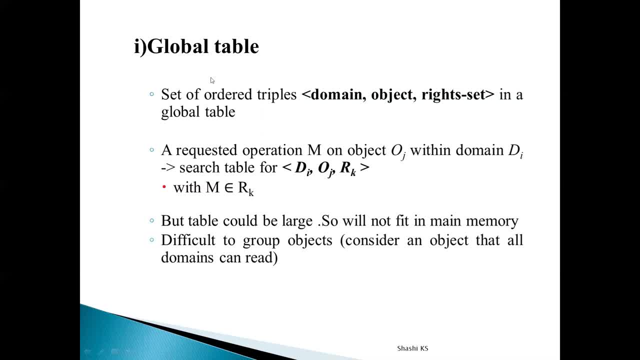 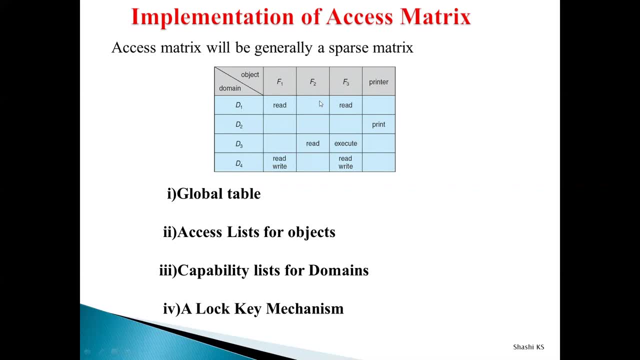 Okay, What is the basic concept of all these implementations of access metrics is, what is the basic requirement for us is, let's say, a process wants to do some particular operation on a particular object, on a particular resource, Whether I should, whether the way I should allow the process to do the operation, or it should be. 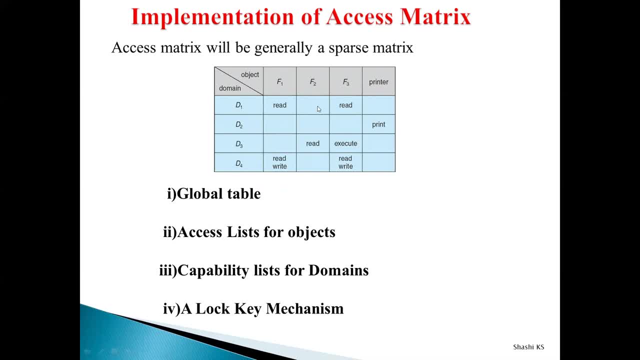 denied The record. That is the basic summary of all of our implementation. All of our implementation should provide me a solution to this problem. If a process wants to request- uh, if a process requests to perform some operation on a particular object or on a. 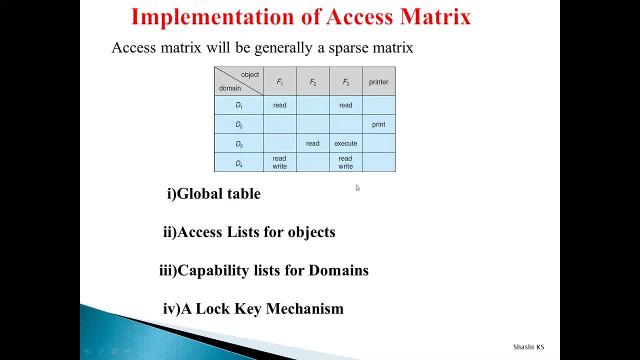 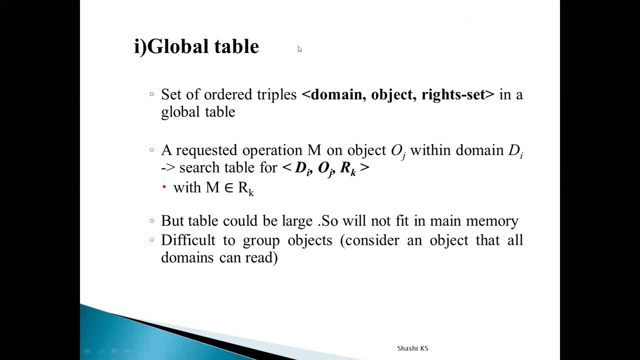 particular resource, whether the way I should allow it or not. that is, that should be the final answer to my question. that should be answered by all this for implementations. So let's see about them. The first one is the global table. in this global table implementation, it maintains: 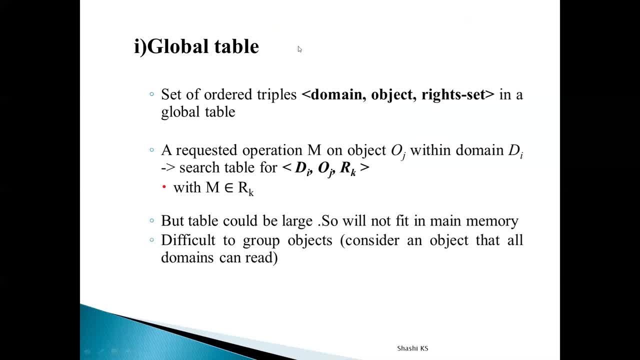 it is nothing, but it is a simple implementation of access metrics. I can say so here. we maintain a set of ordered triples. Every entry in the global table contains a set of ordered triples. That means it maintains three types of information. What is this information? 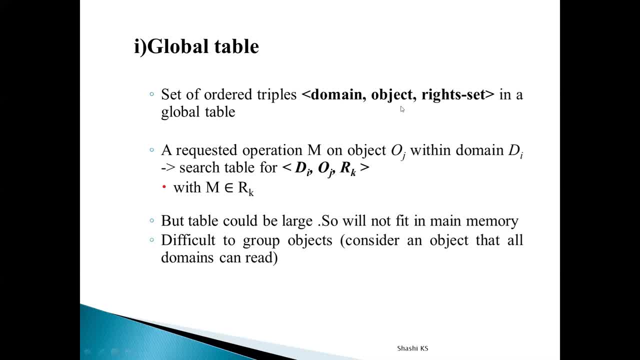 It maintains the domain name. It maintains the object name and the right set. What does it mean? Everything in the access metrics is there in the global table, In each entry of the global table, the domain name, that particular objects which can operate on the domain and separately. 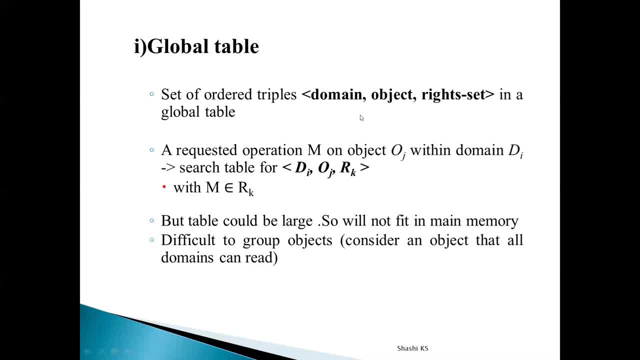 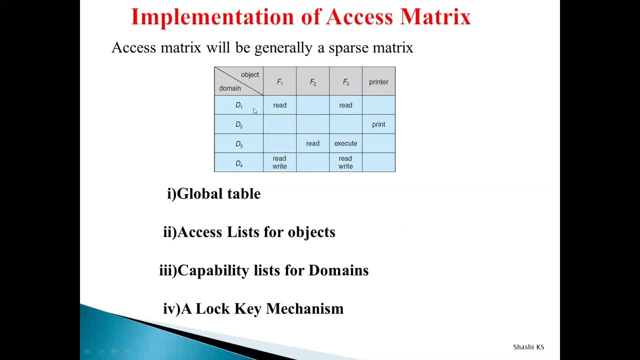 not together. Okay, If. if let's say in this example, in domain D one the object F one and the object F three can operate in domain D one, So separately entries will be there in the global table How it will look like: D one comma, F one comma read and one more entry will be: 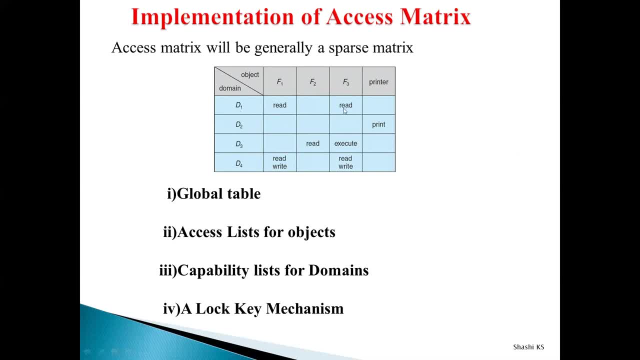 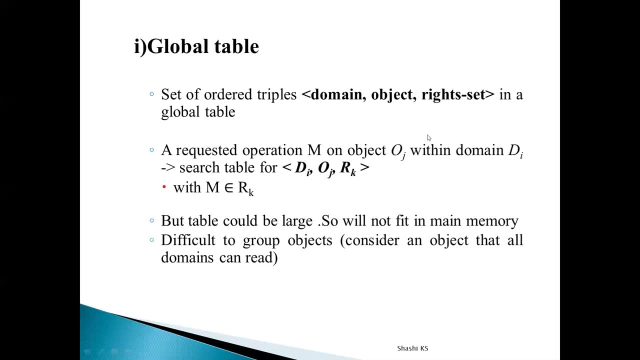 there in the global table, which will look like D- one comma, F- three comma. read So like that: for every object in every domain, separate set of ordered triples will be maintained in the global table. Okay, Now the entries are maintained and entered in the global table. 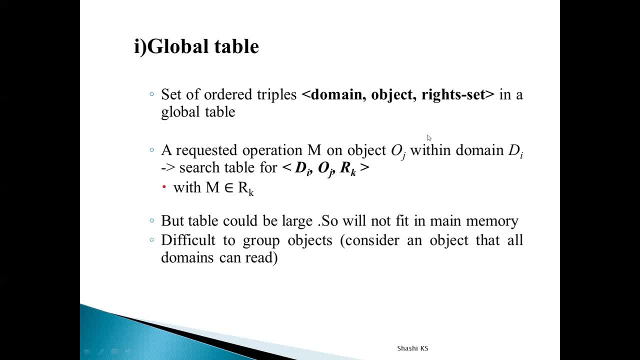 Now, then, how we are going to take decisions based on this global table. Let's say a process request to perform an operation- Yum, Okay, That operation young should be there in the rights set of the particular object. Let's say one process P one wants to perform. 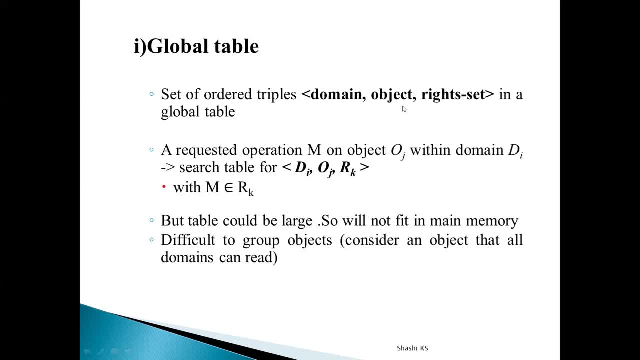 The read operation on object O one. Okay, Then the OS will check if the read operation is there in the rights set of the particular object O one in that particular domain. domain can be anything. It can be D one, D two, D three, four, before, like that. 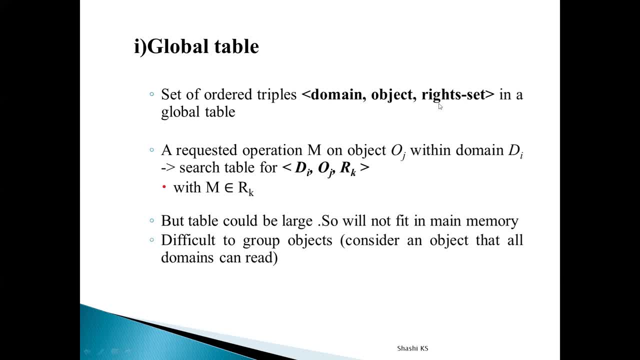 So it will check. the OS will check whether the particular read operation is there in the right set for that particular object O one. If it is there, then the process will be allowed to execute the operation. If it is not there, process will be denied the request. 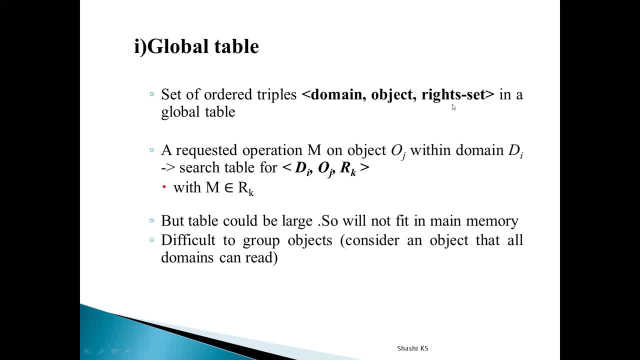 Okay, That is such a very simple implementation. Uh, the process will be denied and an exception or error condition will also be raised because the process is not allowed to do that operation in that particular domain for that particular object. You can. you could have also experienced this when you try to do a right operation on. 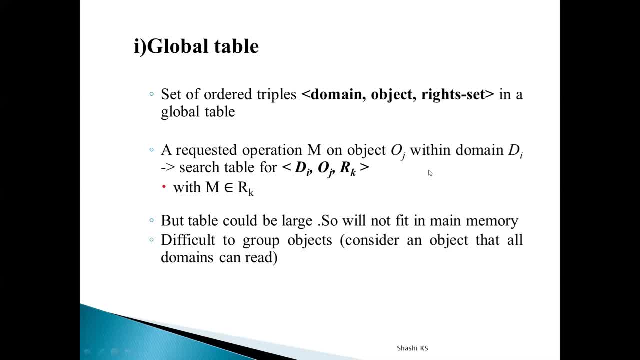 a file And if that particular program does not have that access, an exception will be would have been raised in your programs. Okay, So this is your global table implementation And if you see the advantages, as I already told, it's a very simple implementation. 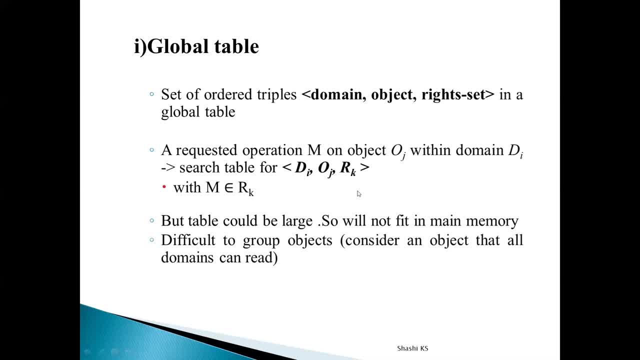 That is the advantage, The disadvantages your global table is going to contain, for all the individual objects, Um, it is going to contain the list of all the right set for all the objects in all the domains. Okay, So the resultant table is going to be large because, separately, 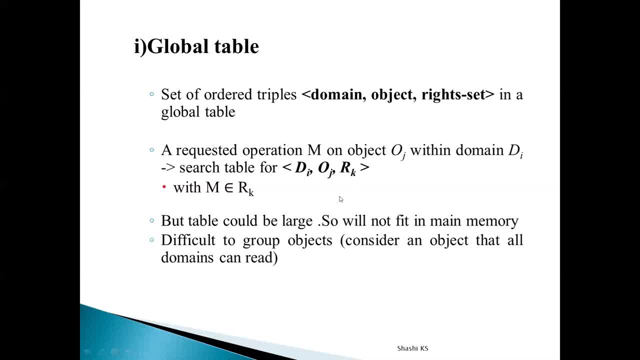 it's going to store information about all the objects, all the domains, in separate entries. So, uh in case, if you have too many objects in your uh system, then the table will be large So you cannot fit it into main memory. 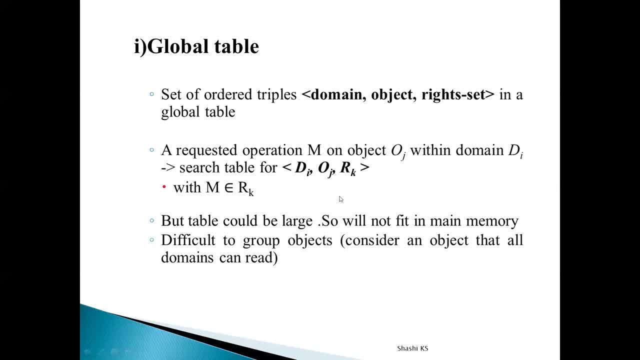 So you need to say, store it in secondary memory, and then you have to make use of virtual memory concepts to bring the required information into the main memory. So that is one disadvantage. Another disadvantage is sometimes you may have some special groupings of objects. 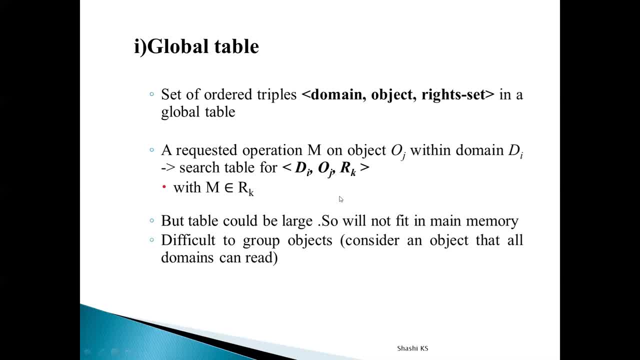 or domain, Say for example: uh, you may have a particular file which can be read in all the domains, Okay, By all the processes, in that case it's a special grouping, but still I cannot take advantage of that special grouping. 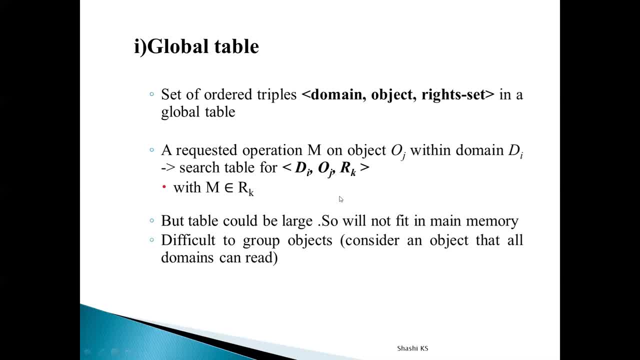 and I cannot reduce the number of entries in my global table. Number of entries in my global table will always remain the same, irrespective of. this is a special case where I have a chance to reduce the number of entries, but still I cannot do that. 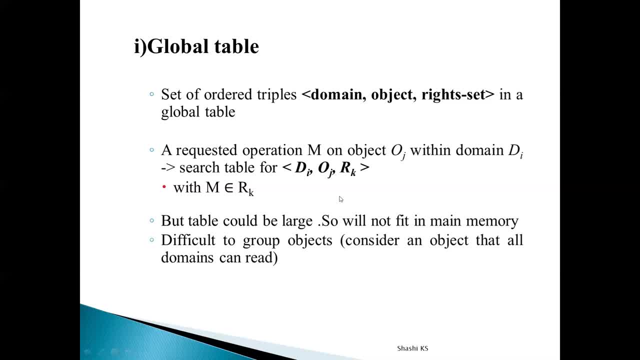 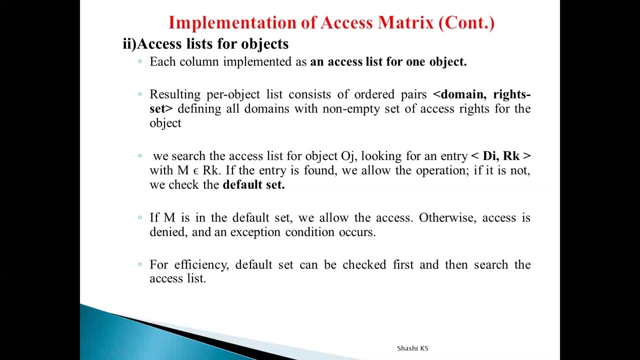 So it is difficult to take advantage of the special cases of special groupings of objects or special groupings of domains. So that is about the disadvantage of this Implementation. Next we will move on to the second type of implementation of the access matrix. 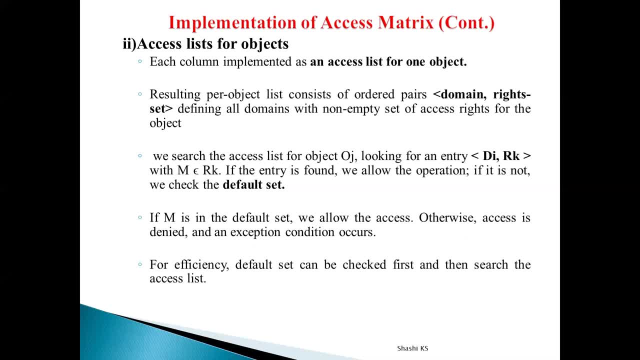 Now the second implementation is called as the access list implementation. We saw about access list, access control list, When we learned about files. this is similar to that access control list concept. here I told you that this. look at the diagram for access matrix. 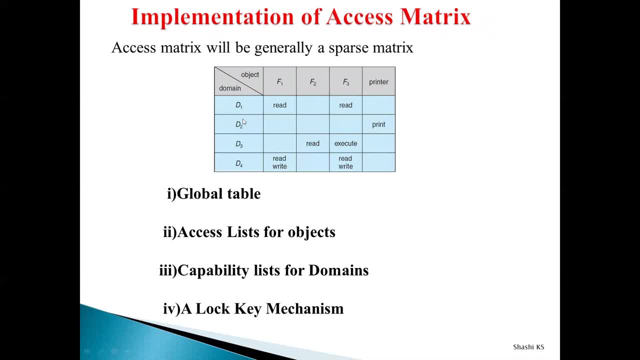 your columns will consist of objects. right, And you are done. my and your uh rows will consist of domains. So in access list, what we do is for every object it maintains a domain and the rights information for the object. 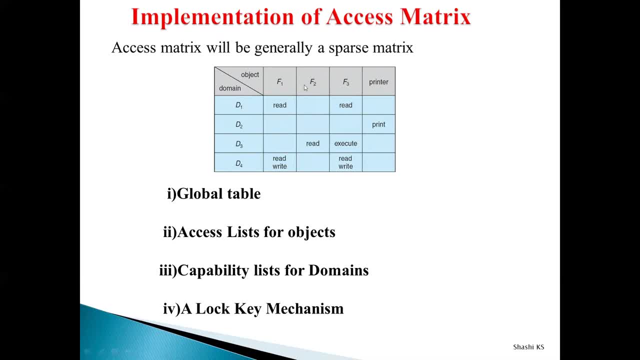 Okay, So your access list is maintained for every object in the column of the access matrix And for every object it maintains a list of domains in which the object can operate and the list of access rates for that object in that particular domain. Okay, 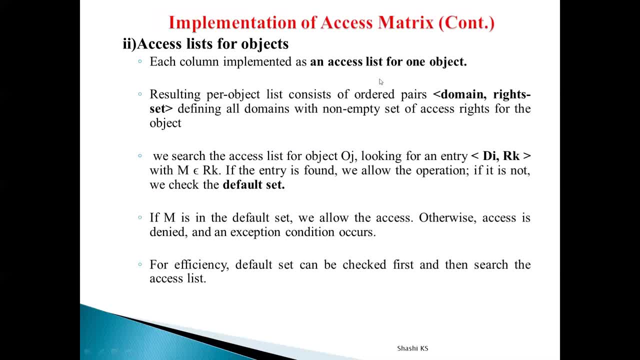 So access list is maintained for each object, And so here it is not a triple, It is a ordered path which consists of the domain in which the object can operate and the right set for that object. Say for example, here in this representation for object F1,: 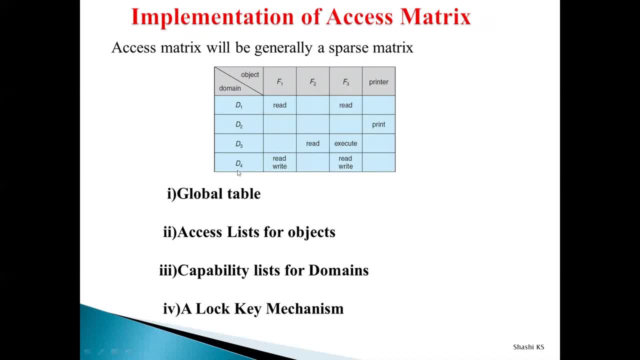 the entry in the access list will be D1 comma read and the D4 comma read comma right. Okay, So for every object, what are all the domains in which it can operate and what are all the access rights which it can perform on in that particular domain? that will be maintained as. 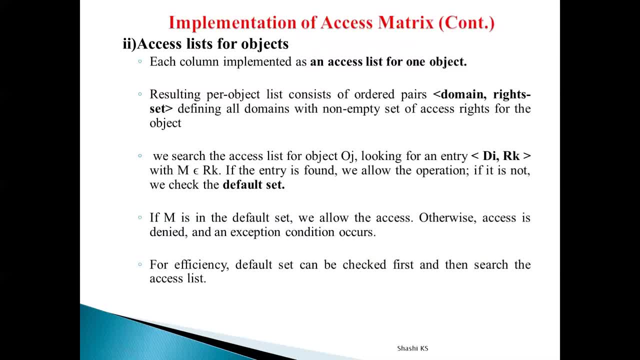 a ordered pair in the access list. Now how are we going to allow the process request or deny the process request in this access list is so: whenever a process request to perform an operation yum, we check whether the operation yum is there in the right set for that object. 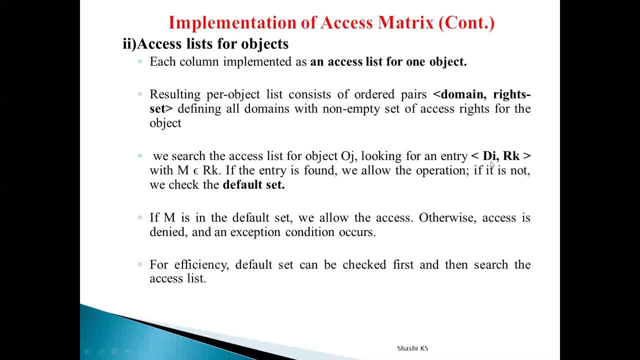 in that particular domain. a process might be in domain D1. it will request to perform some operation. read uh on the um: what for some object for some file, object F1.. Okay, We check for the file object F1.. 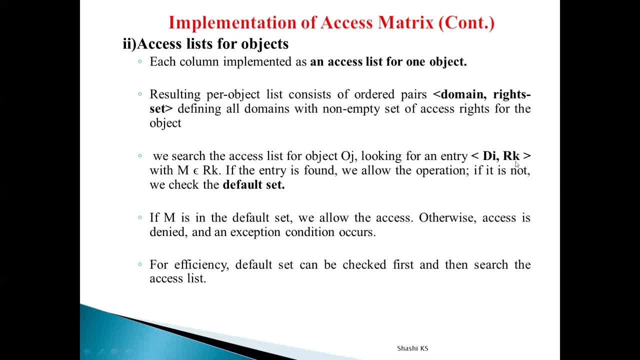 If the read operation is there in the right set for F1.. Okay, If the read operation is there in the right set for that object in that particular domain, in that particular domain, we allow the process to do the operation Now um. 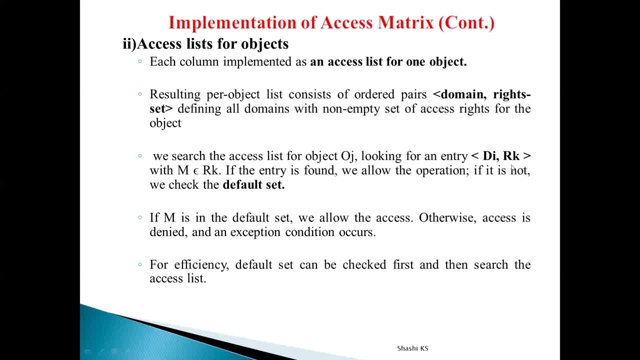 if that read operation is not there in the right set. instead of not allowing the process, what we do is we also have another set called as the default set. Okay, Default set is nothing, but it contains a default set of access rights for every object. 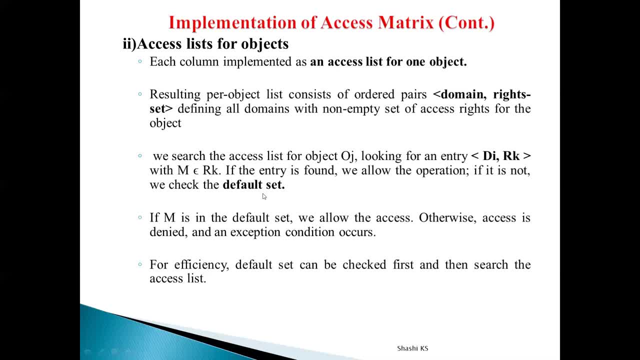 Okay, It also maintains a default set which contains a default set of access rights for every object. So if it is not there here, we check whether, whether the right, whether that operation is there in the default set of access rights for that. 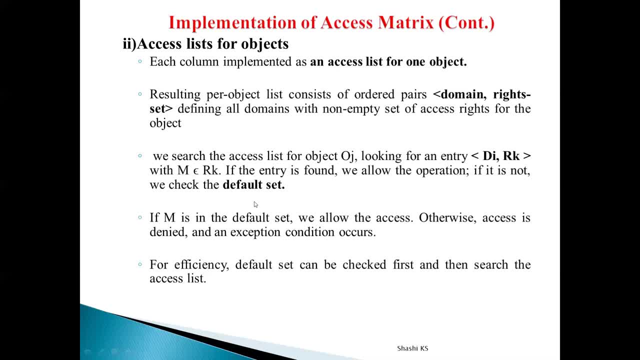 particular object. So there are two possibilities here. right, That operation which I'm searching for might be there in the in the default set of access rights. So if that operation which I am searching for is there in the default set of access rights, 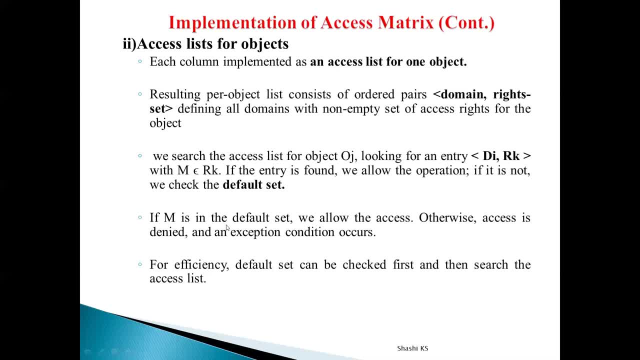 then I allow the access. If the, if it is not there in the default set also, then exception or an error condition will be raised. So here uh, first we are checking the access list and then we are checking the default set. 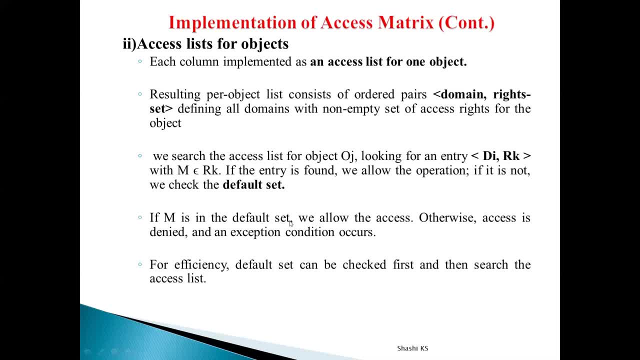 We can also do the vice versa: We can first check the default set and then we can check the access list because, uh, for efficiency purposes. So that is about the second type of implementation of access metrics, which is nothing but your access list. 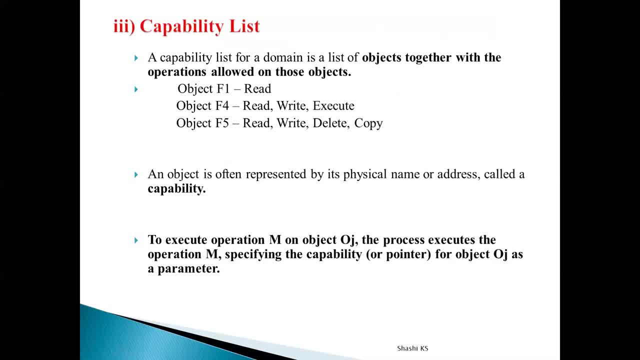 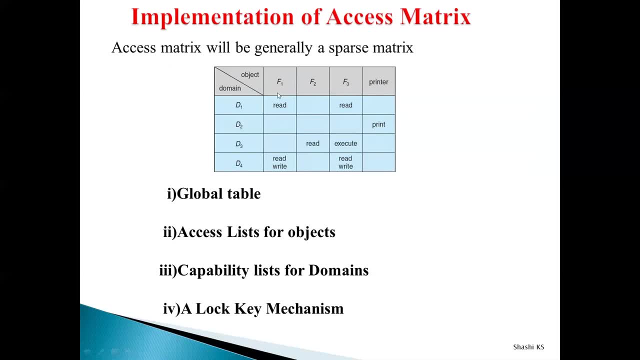 The third type of implementation of your access metrics is called as capability list. Again, come back to our access metrics representation in access list. for every object We maintained the domain name and the operation information for that object right. The reverse is done in the capability list. 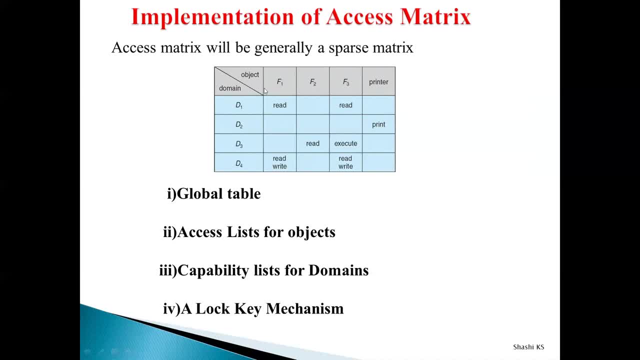 Okay, For every domain we maintain the set of objects and the set of operations which can be performed on the domain. for domain D1, the set of objects are F1, read and F3- read for domain D2.. It is printer come up. print for domain D3. 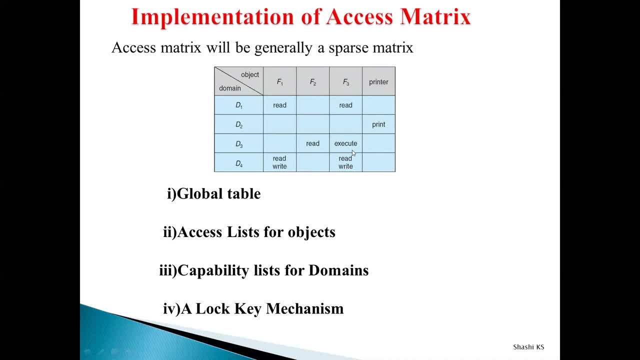 It is F2- read and F3- execute. like that We maintain the set here also in capability list, Also domain wise, we maintain the list of all the objects and the set of all the operations which can be performed on the object. Then that is called us. 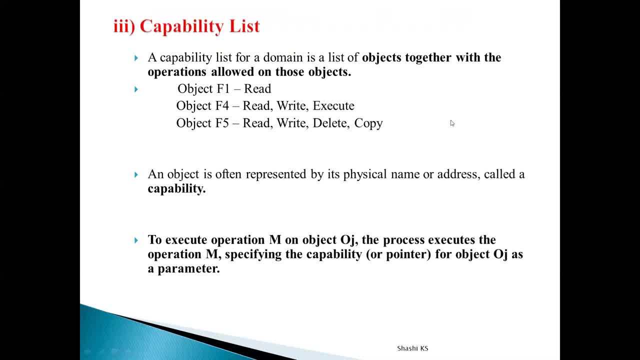 Capability list. Okay, So if I maintain, for every object, if I maintain domain comma access rights, it is called access list, And for every domain, if I maintain object comma access rights information, it is called us capability list. Okay, That is what it has been written here. 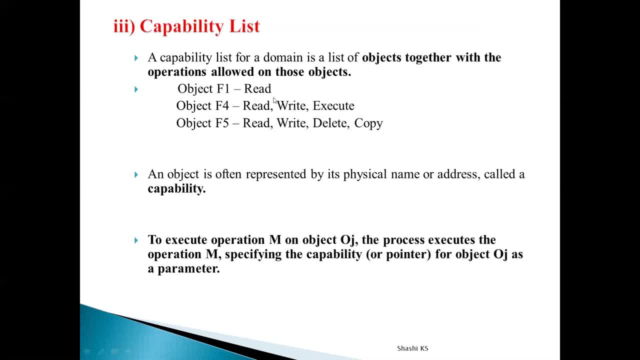 Uh, so for domain D1, I can write in: the domain D1 capability list may contain entries like F1 comma read. F4 comma- read write execute. F5 comma read write delete, copy, like that. So for every domain. 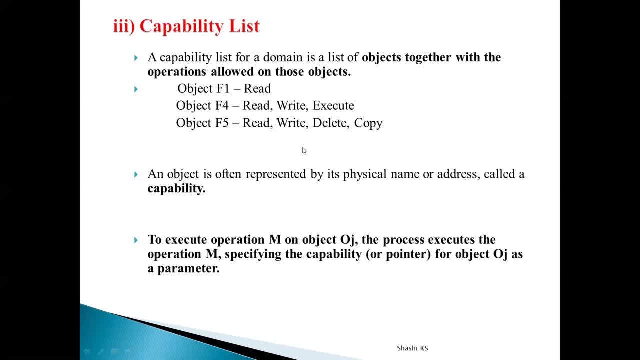 it maintains a list of all the objects and the type of operations which can be performed on the object. But one thing which has to be noted here is: um, here, every object, how to represent objects. So here it is. Capability list is going to store the object information that every 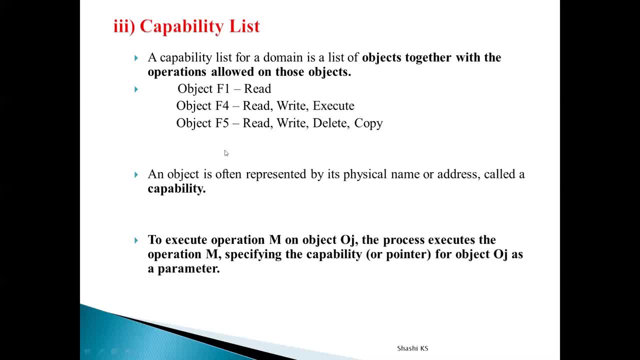 object has to be identified. to identify every object will be represented by its name or by, uh, the unique address. Okay, That address or the name which we use to represent an object here is called as the capability. Okay, The name or the address. 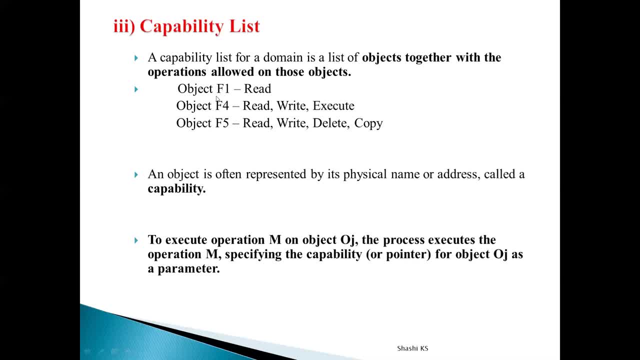 which we use to represent a particular object in a particular domain is called as capability. Okay, And the important point to note here is if a process wants to do some operation on a particular object, some particular object, let's say if a process 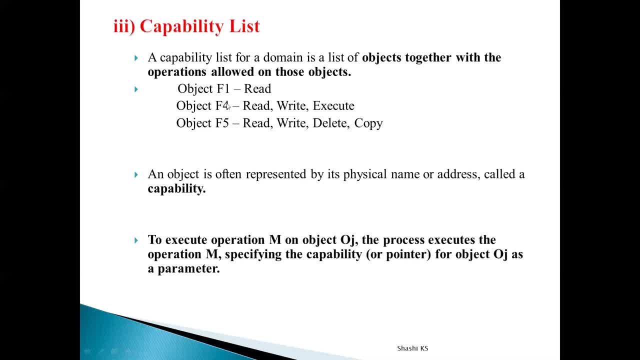 P1 wants to perform some operation on a particular object F1,, then the process has to just uh, if process has to just possess the pointer or the capability for that particular object. if a process wants to do read operation for object F1,. 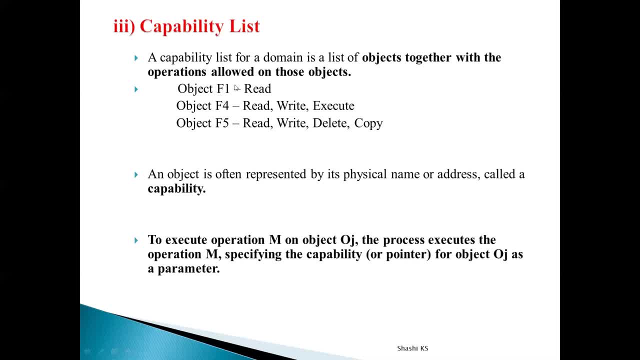 it has to possess the pointer address or the name or the, or we call it as capability. So the process should process the capability for the objective Simply. If the process possesses the capability, it will be able to do the operation. If the process 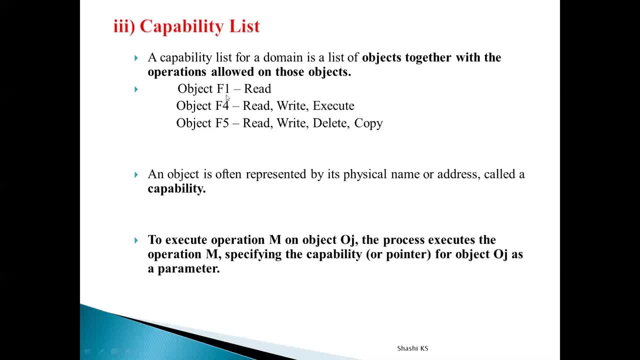 does not possess the capability, it will not be able to do the operation. Okay, So that is how it operates. So it is slightly different from our previous two methods. here, every object and its access rights will be maintained in the capability list. 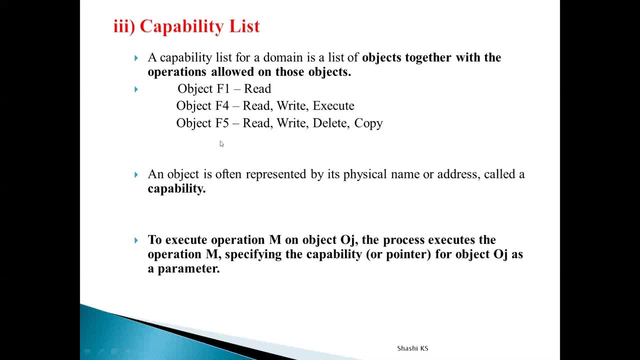 And every object will be represented by object name or object address, So that object name or address is called a capability. So if, uh, if a particular process wants to do an operation on an object, it has to know the name or the address of the object. 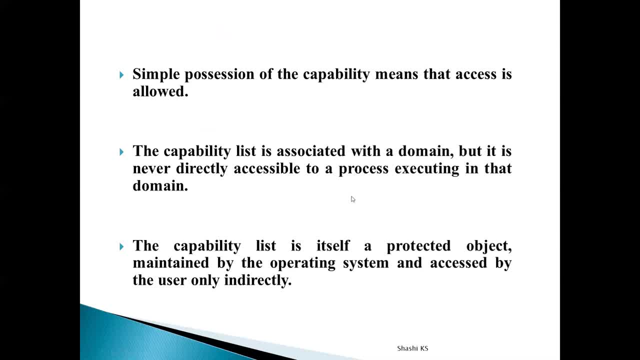 So simple, position of the capability means that access will be allowed for the user. So but then you can see that obviously, simply, if the process possesses the capability, the process would be able to do the operation on the capability. So that's why. 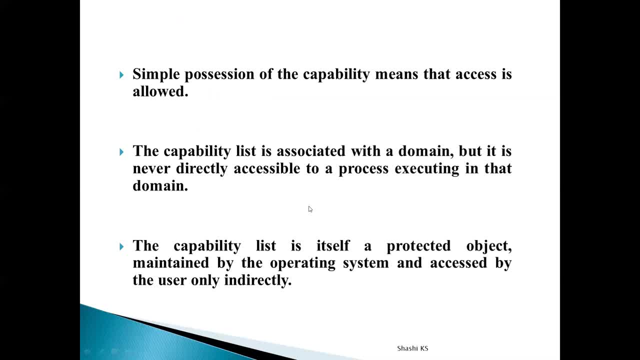 but then then we have to protect the capability. It cannot be freely accessible to all the processes, right? So for that reason here the capability list is maintained as a protected object. The capabilities and the capability list is maintained as a protected object. 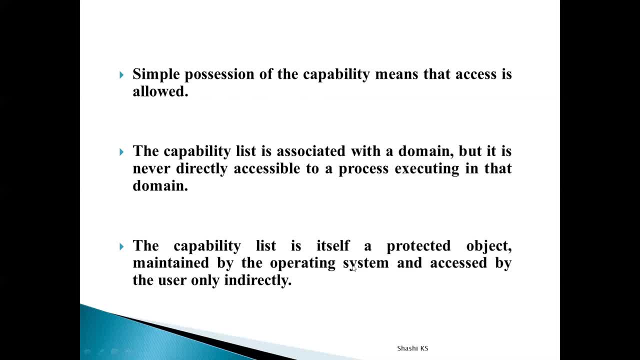 And it is maintained by the OS only does not directly accessible in any address space which is directly accessed by the programs or by the users. because if the user has the capability, he can do any operation on any object right. So for that reason, 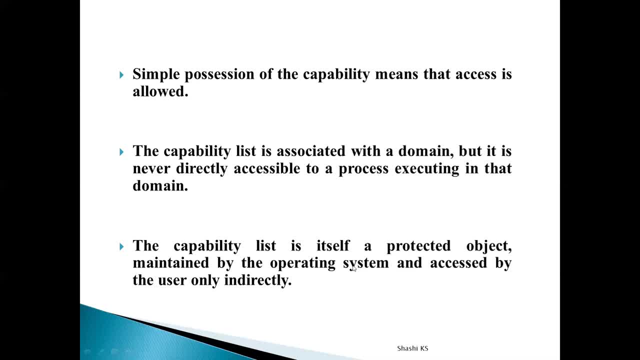 capability is not freely accessible to the users and it's not stored in any address space which the user can freely access. it is stored in only the address space which is belonging to the operating system as a protected object And and the capability list, as I told you. 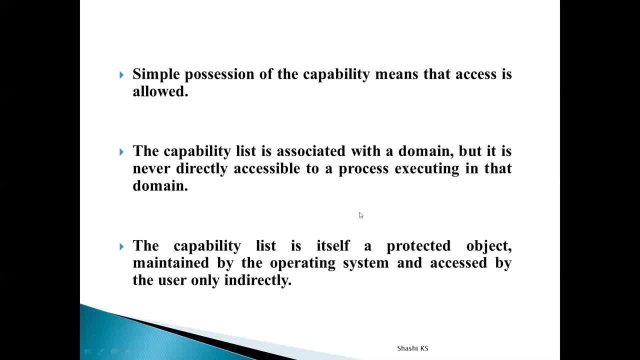 capability list is associated with the domain. for every domain, What are all the objects which can operate on the domain and what are all the operations which can be performed on that object? That list is being maintained, So it's. it is associated with a domain only. 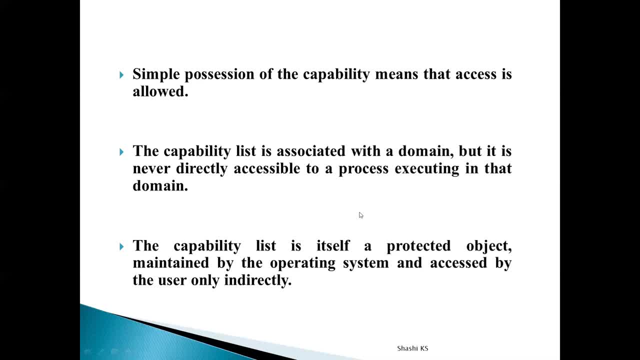 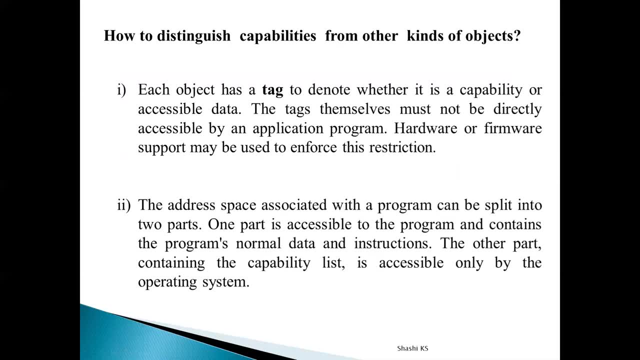 right. It's not associated with any particular object or any particular process operating in the domain. So that is about capability. So from this you can understand that capability is nothing but object name or an object address which is associated with a particular domain. 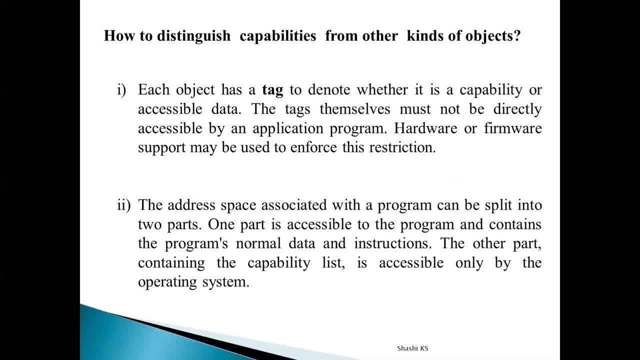 So but then? so here, capability is also an object which is nothing but an object name or an object address which is associated with a particular domain. You can also have some other kinds of objects in the system, Say, for example, different data types. 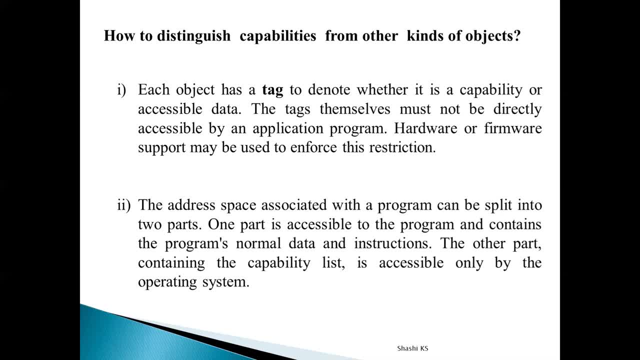 your integers or your floating point values or your double values. the other kinds of objects may also be there. So how, how are we going to distinguish the objects representing the domains which we call here as capabality, how we will distinguish our capab登 from other kinds of objects? 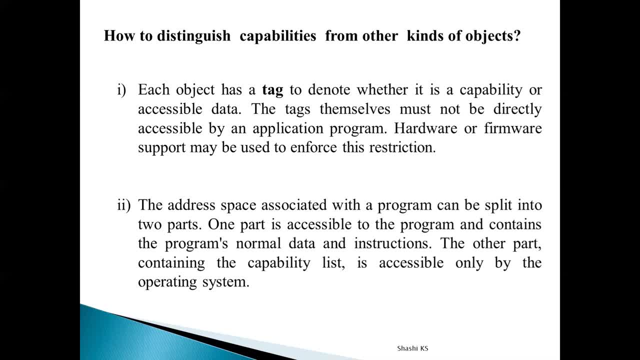 So there are basically two types of ways to do that. one way is, for every object we can have a field called as tag. Okay, So that tag field will indicate whether it is a capability object or whether it is a regular other accessible object, because capability means it should not be accessible by programs or processes. 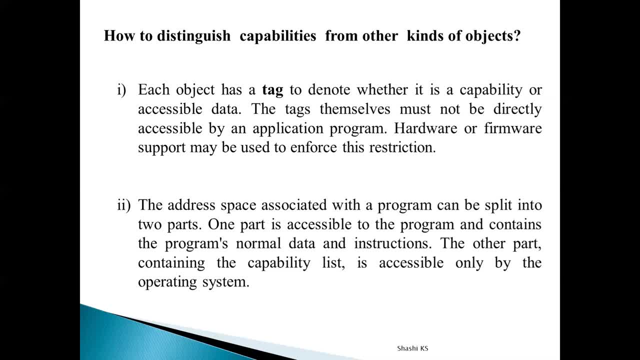 but other kinds of data can be accessed to others by processes, So we need to differentiate, otherwise every process will be able to access the capability, So that's why we maintain a tag which will store the information about whether the object is a capability or any other accessible object, And this can be implemented. 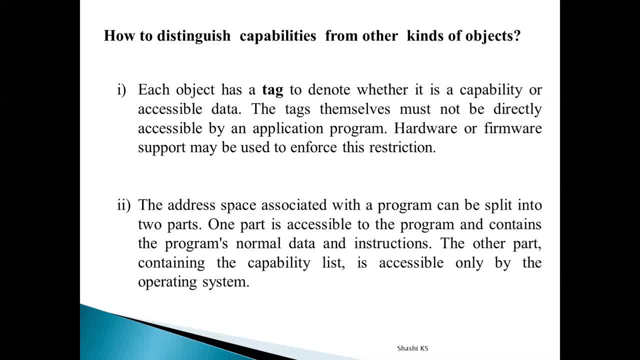 with the help of hardware or firmware support by the operating system. The other way is we can split the address space of a program into two parts. One part of the program may store the regular instructions and the data of the program, And the other part of the 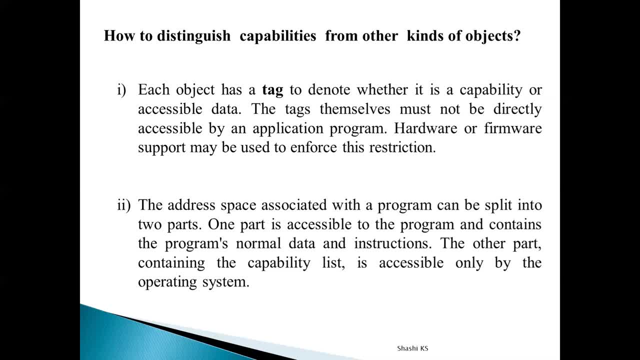 program may store the capability list So that the other part of the program will contain the capability list and that is accessible only to the operating system. So that is how we can. that is two types of ways in which we can distinguish capabilities from other. 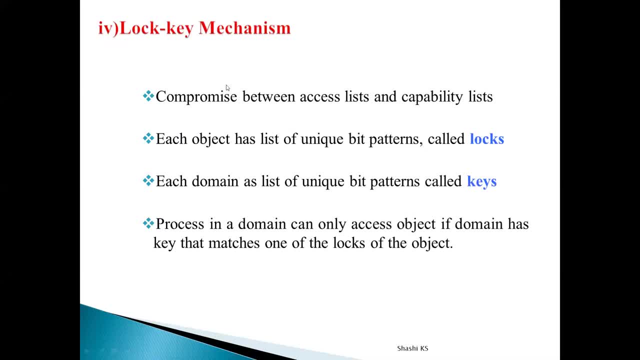 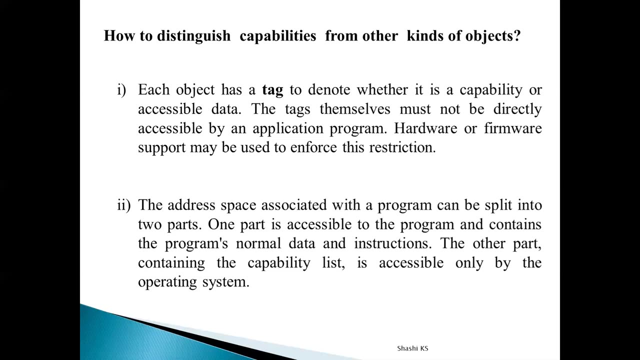 kinds of objects. The fourth type of access matrix implementation is called as the lock key mechanism. Now, this lock key mechanism- So in the previous method- this example is Mac operating system- uses a capability based protection system And here this lock key mechanism is just an. 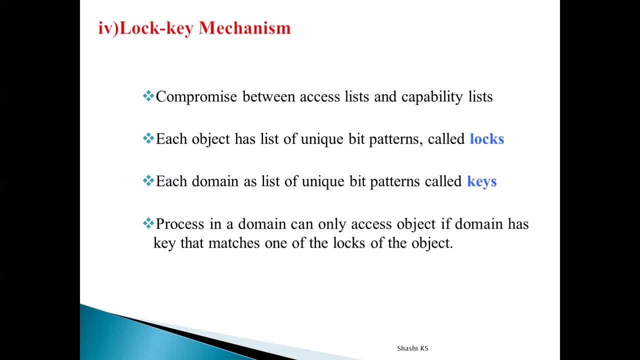 in between between the access list method and the capability list method. Here what we do is we know that the rows of access matrix contains domains and the columns of access matrix contains objects. So each domain contains the unique bit patterns called as the keys Understand that domain is going to contain unique bit. 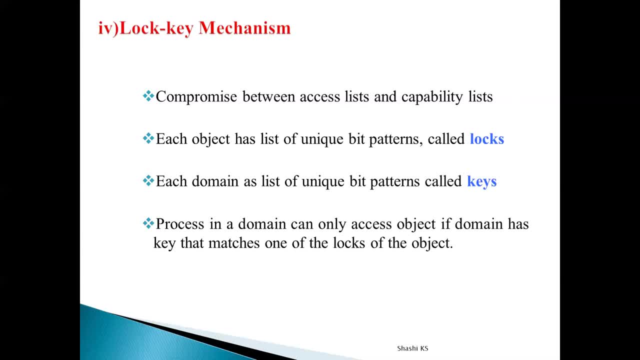 patterns and that is called as keys. Keys are maintained in the domain And each object has a list of unique bit patterns called as the locks. So locks are going to be maintained, The patterns, bit patterns maintained in the object of all this logs. Okay, Let's say 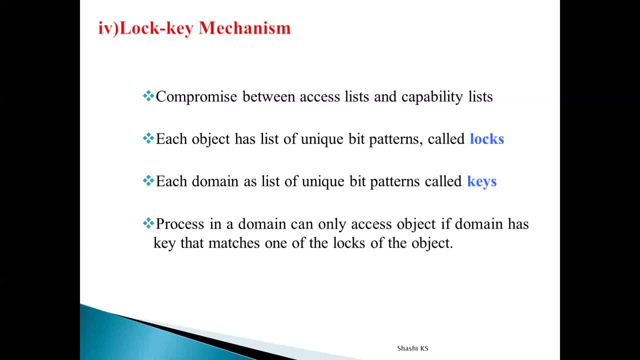 a process in one particular domain may wants to access an object, So the process will be having the locks, your object may access an object, So the process will be having the locks lock and for uh, in order to get the key for accessing that object. the key is going to be: 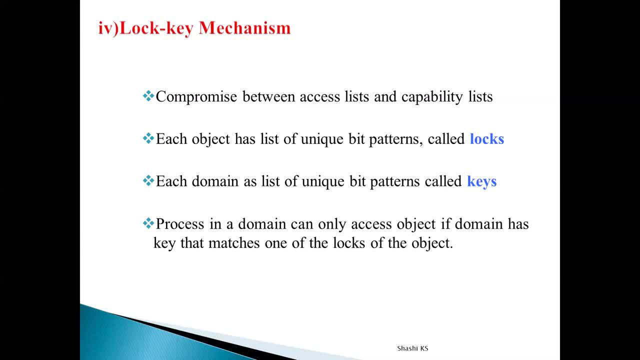 there in the domain. okay, so if the key present in the domain matches with the lock present in the object, matches with the lock which is possessed by the object, what is the meaning of that? the bit pattern which the object is having should match with the bit pattern which is present in. 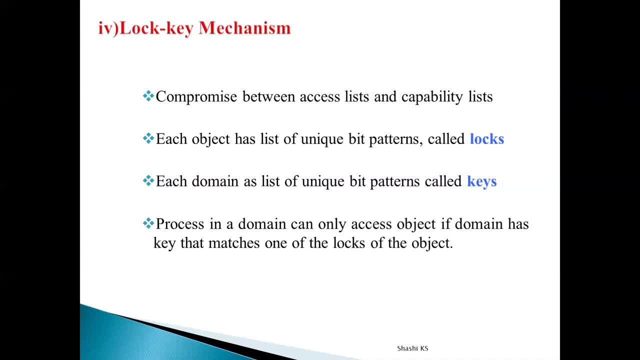 the domain object may be having several locks for several, um, for several domains, right? so the bit pattern, one of the bit pattern, which is which is possessed by the process, should match with the bit pattern present in the domain. that means, in other words, the object should, in other words, the 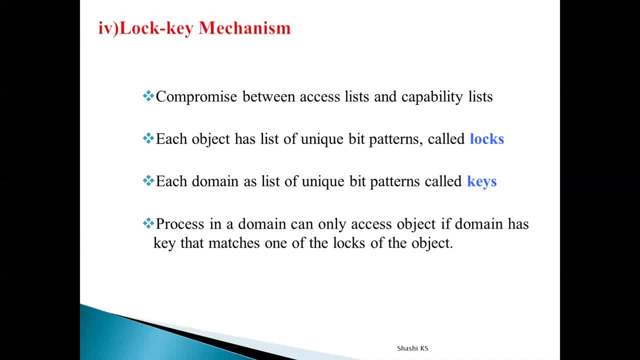 process should possess the bit pattern or the key for opening the lock for the object in the domain. okay, if the process has the key or the bit pattern for opening the lock for the object in the domain, then it will be able to access the object. say, for example, if you have a particular process, p1, it wants to. uh, it wants. 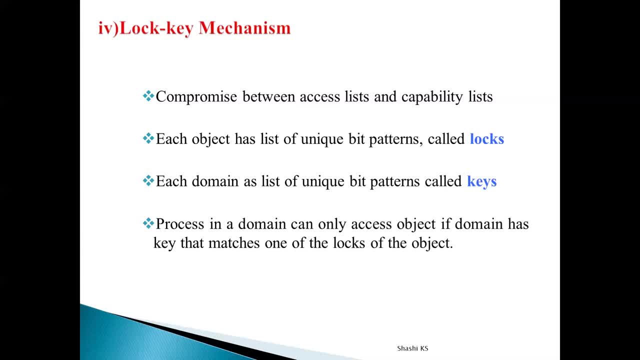 to read a file f1. okay, so it needs to have. if it wants to read the file f1 in this lock key mechanism, it needs to have the key for the file f1. where will it have the key? if the file f1 is in domain d1, the domain d1 will have the key. key is nothing, but it's a unique. 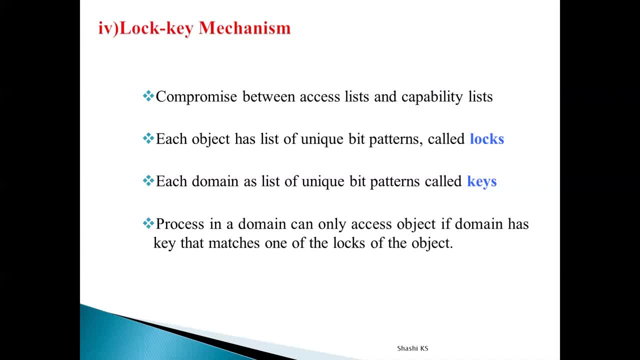 bit pattern and the process p1 will also have a unique bit pattern. the unique bit pattern present in the process is called lock and the unique bit pattern present in the domain of the file f1 is called key. both of them should match, if only. if the both the bit patterns match, then the process 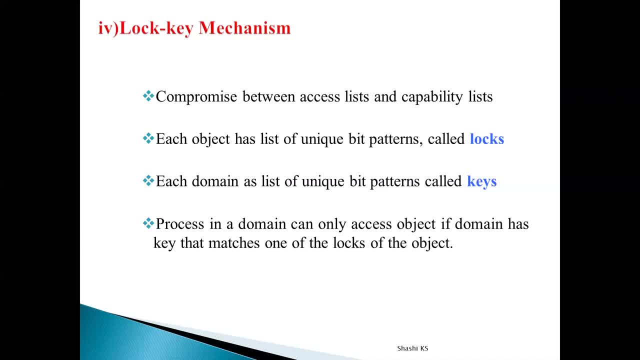 will be allowed to perform the read operation on the file f1, otherwise it will not be allowed. so this is called as the lock key mechanism, uh, so here also, uh, the list of keys, obviously with if key is there, any process will be able to access any particular object. right? 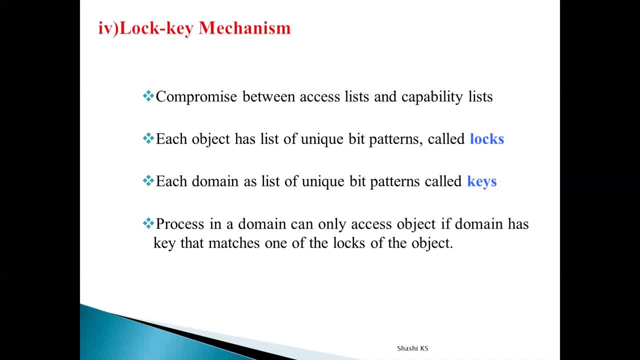 and do any operation. so just like capabilities, the list of keys for a domain must also be managed by the operating system. here, just like capability list is managed by the operating system, the list of keys must also be managed by the operating system on behalf of the domain and users will. 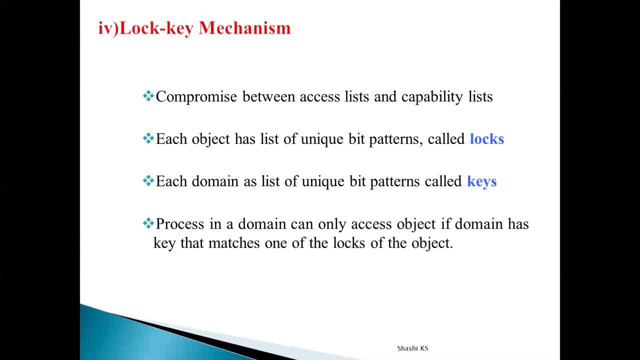 not be able to examine the list of keys or examine the list of locks, or they may, they will not be able to do the operation on behalf of the domain. so this is called as the lock key mechanism: be able to modify the keys or the locks. so in this way, protection is enforced in your lock and key. 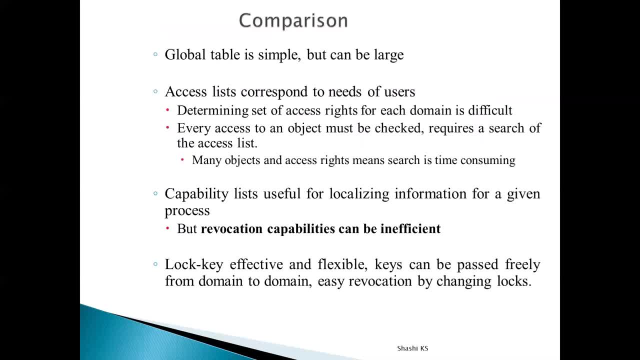 mechanism. so if you compare the different types of, so these are four different types of access matrix implementation. what are they? global table, access list, capability lists and your lock and key mechanism. so, if you compare the different types of implementations, the first implementation, global table implementation, is simple implementation, but then i, as i told you, every information is. 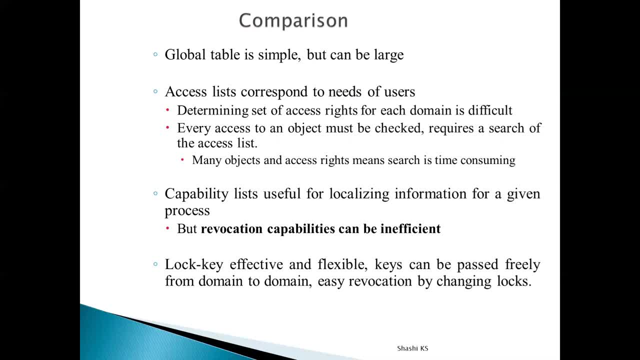 entered into the global table, so global table becomes large and so we need to maintain it in the secondary memory. so that is a disadvantage. if you compare the access list directly, the it is maintained by the users, so every right access, right information is decided by the users. 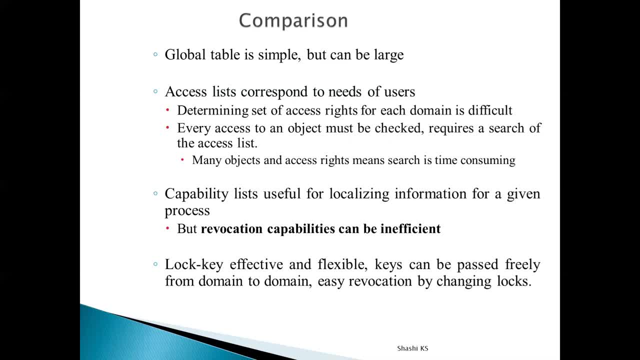 so access. this directly corresponds to the needs of the users. but then the disadvantage here is how to determine what will be the set of access rights which should be there in the each domain and which should not be there in each domain. that is one disadvantage. determining that is difficult. and the second disadvantage is whenever. 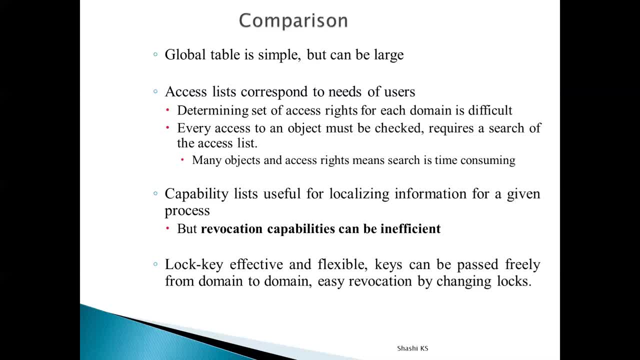 we want to check whether a particular operation can be performed on a particular object or not, we have to search through the entire access list and that is a very time consuming task. the third method is our capability list. in the case of capability list, we know that simply a 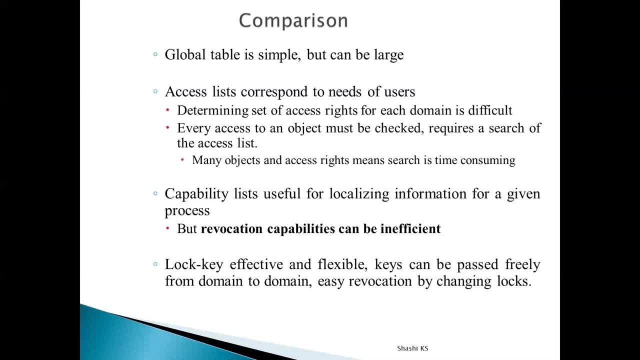 process. if it wants to perform an operation on an object, it has to possess the capability for that. and then to achieve that capacity, we should function to give that capability, like such that right now, let us say, you give a capability for a particular object, for a particular domain, how to? 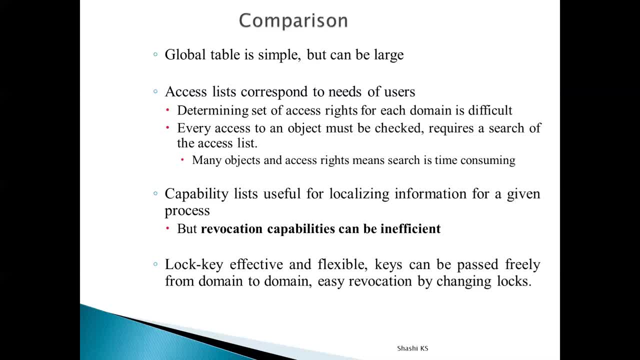 revoke the capabilities you do you give. simply, if the process possesses the capability, it will be able to do the operation and the capability on the object. but then, once you give the capability to a process, how to revoke the capabilities? that is nothing but access rights of executing a particular. 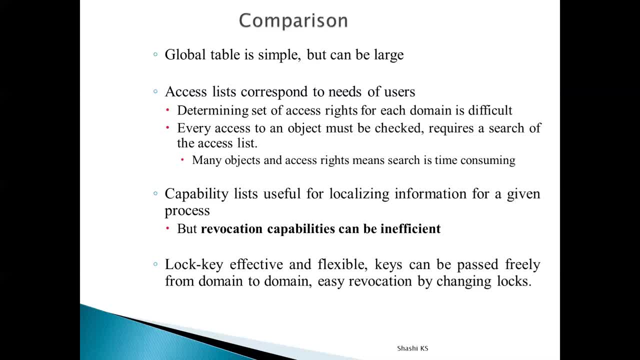 object on a particular domain. it's called capability. so how to capability list method? the fourth method is lock and key method. this is effective and flexible method and you can also pass the keys from freely from one domain to another. and if you want to rework the access rights, how are how can we do it? just, you change the locks, right if the keys are. 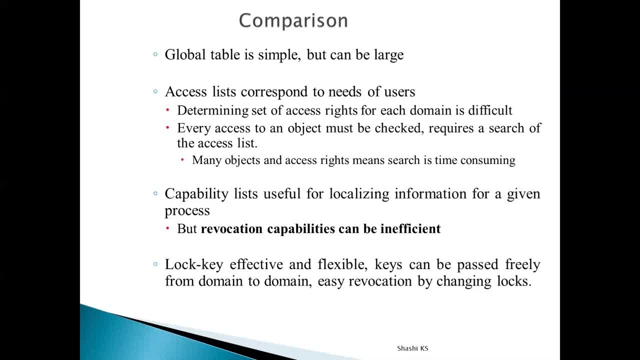 going to be present in the domain. so you just change the locks, which is nothing but the bit patterns associated with the objects. so you just change the locks, you will be able to revoke the access rights. so if the bit pattern doesn't match, the process will not be able to access the 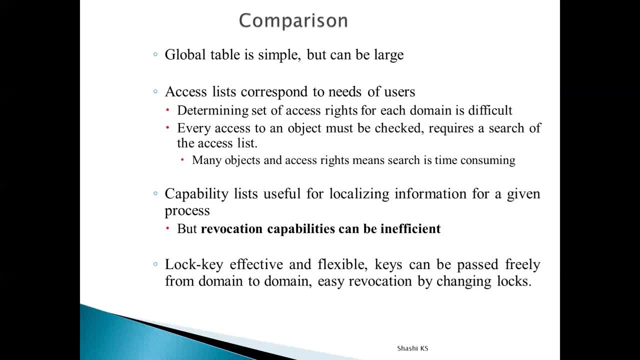 particular object so you can change the locks or you can change the keys and by that you can revoke the access rights. so that is about the comparison of different types of methods. so with this we come to the end of this lecture. we saw about to summarize. we saw about the different. 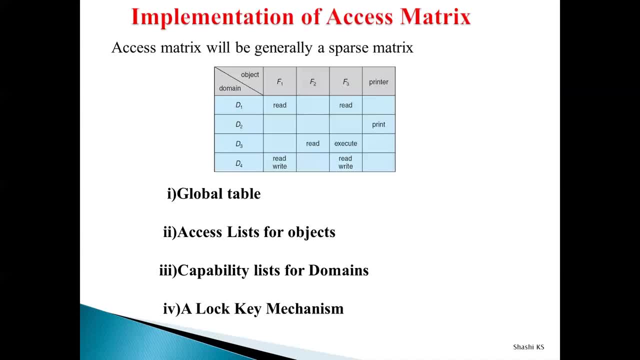 types of methods. so if you want to change the locks, you can change the locks to the objects of access matrix implementation, which is nothing but your global table implementation, access list for objects, capability lists for domains and lock key mechanism. we saw that in access list for every object we maintain the domain for. 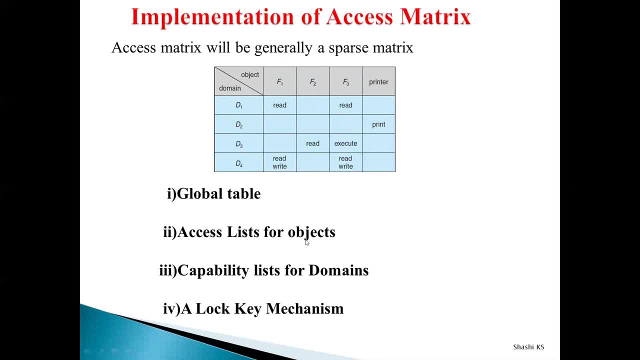 every object, we maintain the domain comma access rights for the object. in capability list for every domain, we maintain the object comma access rights for the domain. okay, and in lock and key mechanism, unique bit patterns are maintained both in the domains as well as in the objects and both should match.